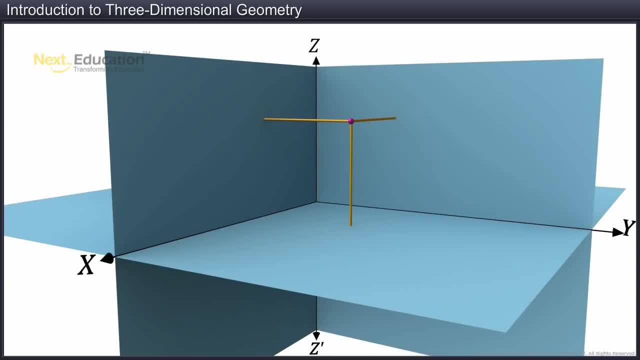 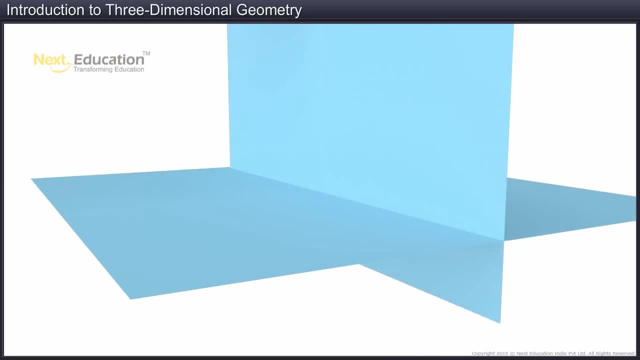 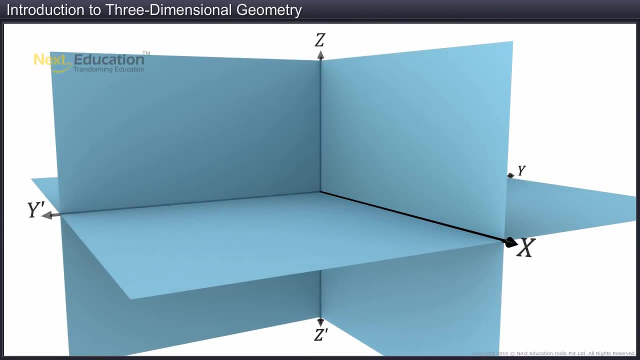 Let's see what these reference planes are and how to locate a point in space. We take two planes perpendicular to each other. The intersection of these two perpendicular planes is a straight line. Let's take another plane, perpendicular to both the existing planes, With the intersection of this plane with the two existing planes. 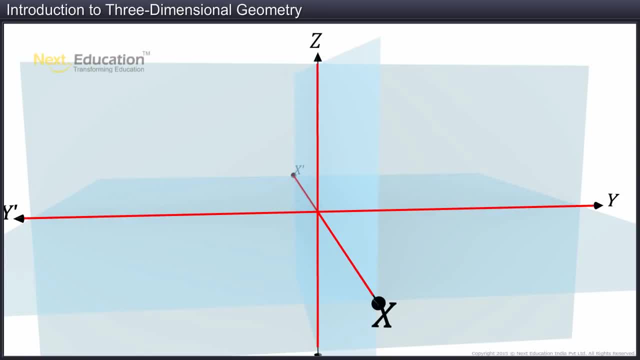 we get three lines mutually perpendicular to each other. These lines are called axes and are named as x, y and z. The point of their concurrence is a point in space. The point of their concurrence is called the origin. The origin is denoted by the letter O. 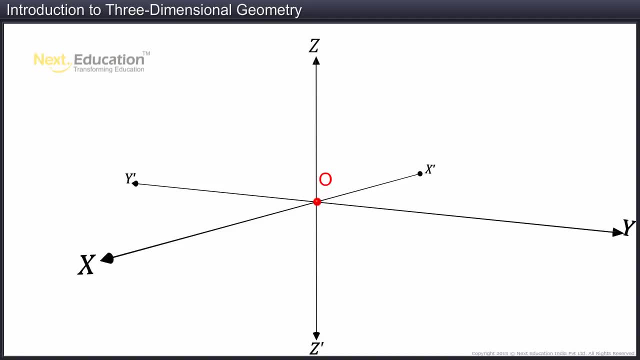 By convention we consider the x- y plane as the horizontal plane. Distances are measured starting from the origin. Distances measured in one direction are taken as positive and in the opposite side as negative. For example, the distance measured from the origin is called the horizontal plane. 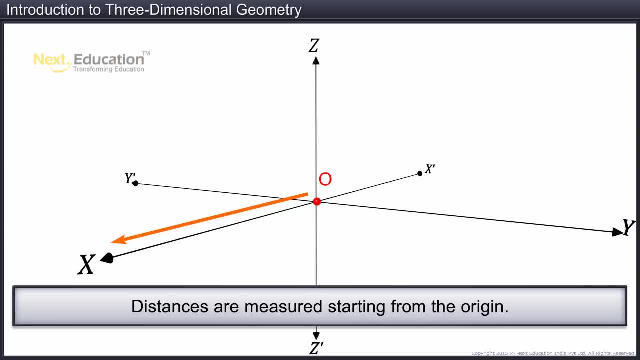 The origin along the x-axis along the direction shown is taken as positive. The distance measured from the origin in the opposite side is considered negative. To indicate this, we assign the symbol x' A similar convention is followed for calculating the distances along the y and z-axis. 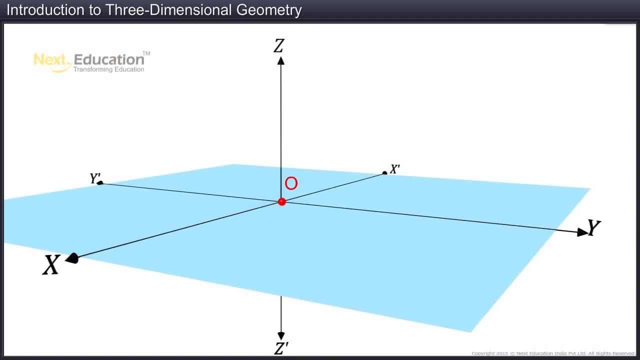 The plane formed by the x and z-axis is called the horizontal plane and y-axis is called the xy-plane. Similarly, the plane formed by the y- and z-axis is called the yz-plane, and the plane formed by the z- and x-axis is called the zx-plane. 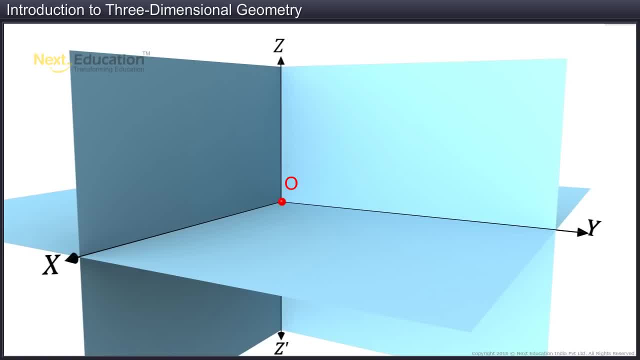 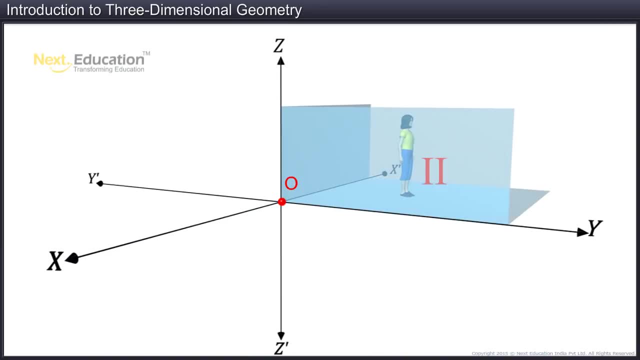 The xy-plane, yz-plane and zx-plane divide space into eight octants. Here x o y z is an octant. This octant is enclosed by the x- y- z-axis. Similarly, the other octants are named according to the axes that enclose them. 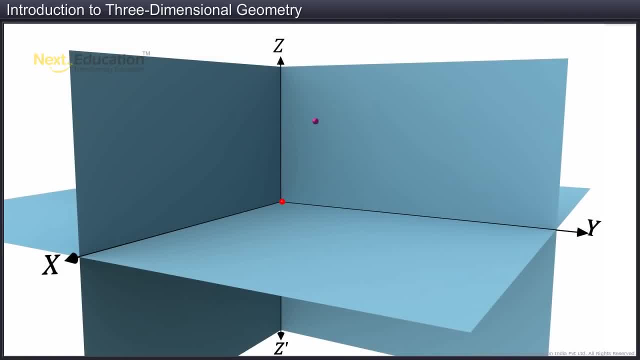 Any point in space is represented with the help of the distance between the two octants. There are also distances that it measures with respect to the planes. These distances are called the coordinates of the point. Suppose we have a point P in space. The coordinates of this point are x, y, z. 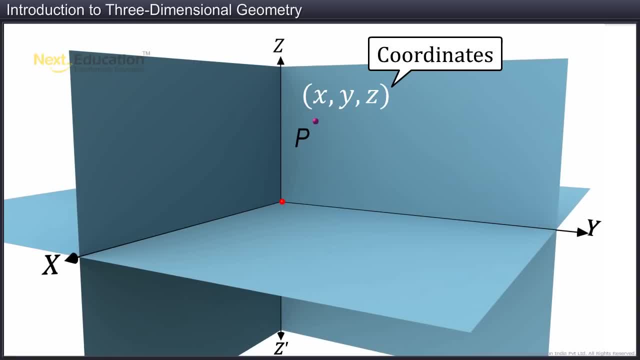 Each coordinate individually indicates the shortest distance of the point from the corresponding plane. For example, the coordinate x, y, z is the shortest distance from the corresponding plane. This coordinate determines the shortest distance of the point from the y- z-plane. Similarly, the y-coordinate represents the distance of the point from the zx-plane. 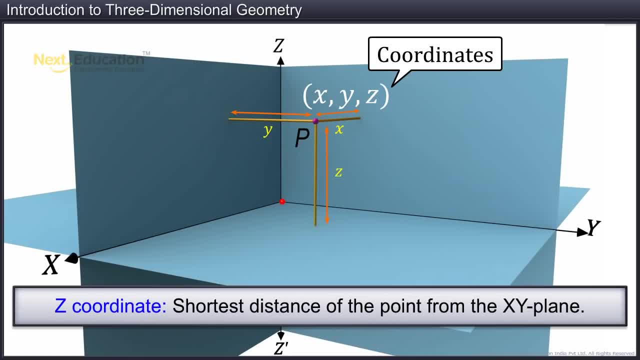 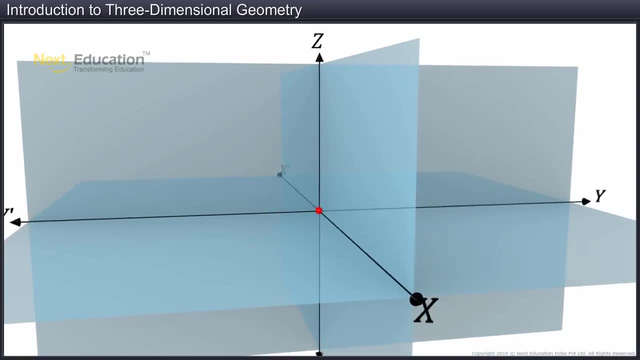 and z represents the distance of the point from the xy-plane. The coordinates of the origin are 0, 0, 0.. Having seen the coordinate axes, we will explore how we use the coordinate axes in locating a point in the coordinate space. 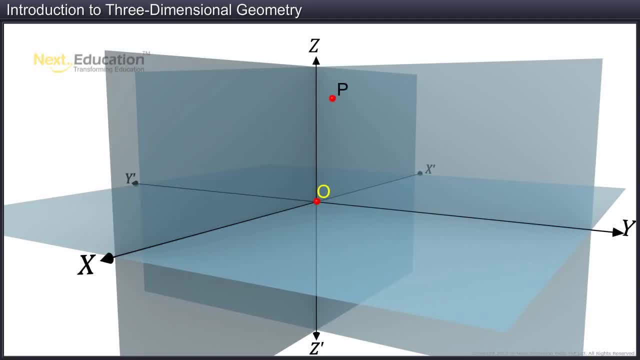 Given a point in space, we can measure its distance from the coordinate planes. Let's see how. One way is to drop a perpendicular on the xy-plane. Let this perpendicular meet the xy-plane at point Q. Then we drop a perpendicular from Q on the x-axis. 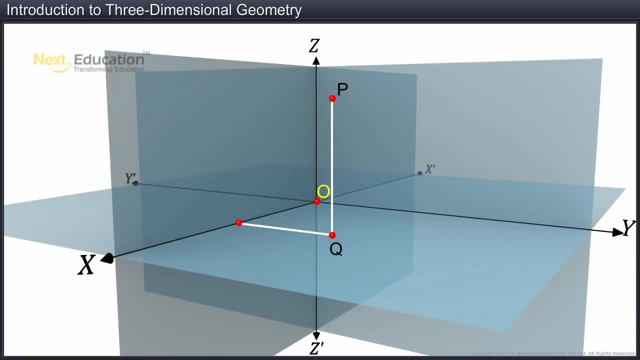 This meets at a point, say R. This meets at a point, say R. This meets at a point, say R. Distance OR is the x-coordinate, RQ is the y-coordinate And PQ is the z-coordinate. 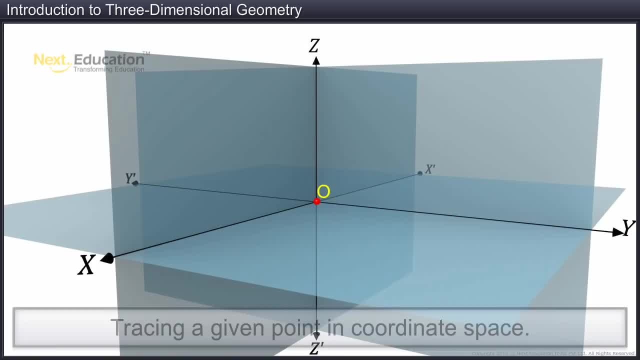 And PQ is the z-coordinate. If we are given the coordinates of a point, If we are given the coordinates of a point, then we can trace the point as shown. then we can trace the point as shown. First we will identify a point. 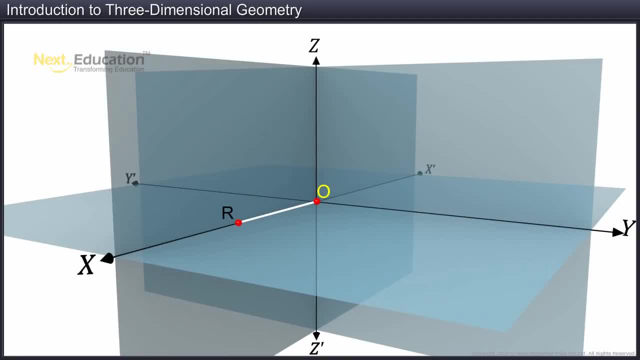 say R on the x-axis, which is at a distance x from the origin, which is at a distance x from the origin. Next, we draw a perpendicular of length y from point R and parallel to the y-axis on the xy-plane. 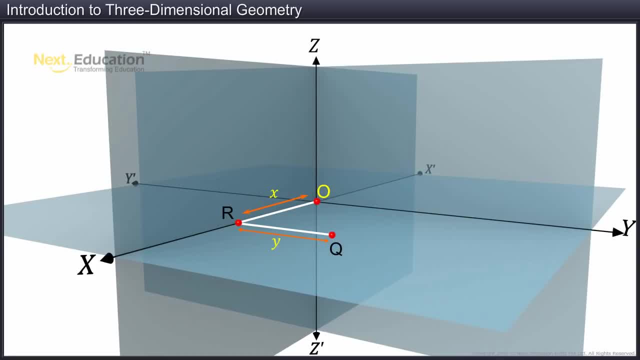 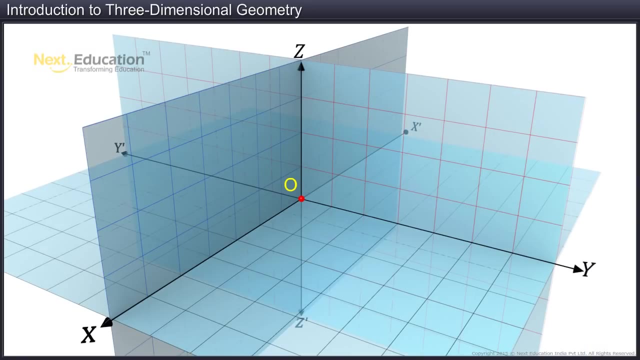 to a point, say Q. Lastly, we draw a perpendicular of length z from point Q, perpendicular to the xy-plane. We can observe an interesting property among the coordinates of the points: Any point that lies on the x-axis will have its coordinates. 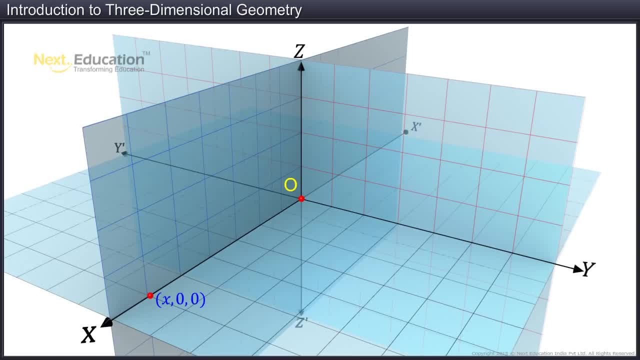 in the form. For example, a point at a distance of 6 units from the origin on the x-axis will have the coordinates. Similarly, the points that lie on the y-axis will have coordinates of the form And the points on the z-axis. 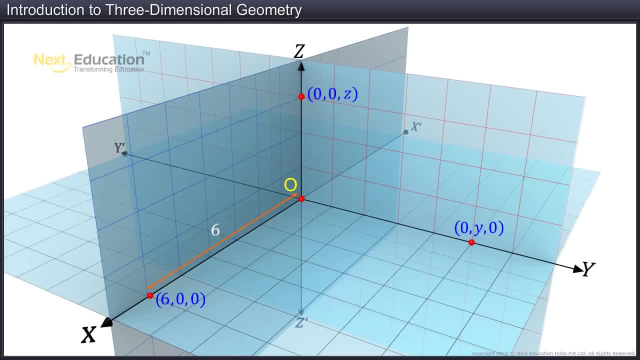 will have coordinates of the form. Here the letters x, y and z belong to the set of real numbers. Any point on the xy-plane will be of the form. Any point on the xy-plane will be of the form Shown. here are some points. 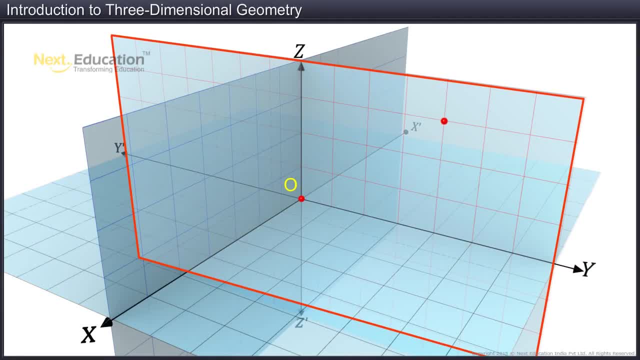 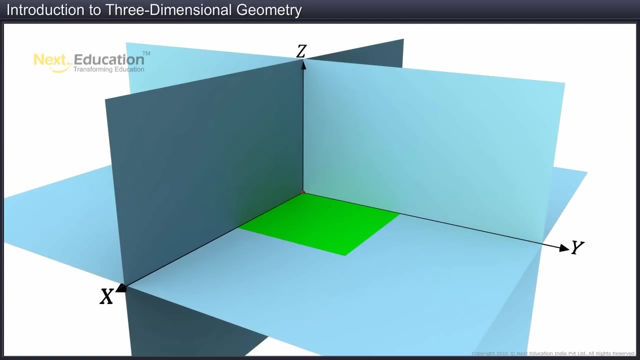 on the xy-plane. Any point on the yz-plane will be of the form and a point on the zx-plane will be of the form. Here the letters x, y and z belong to the form, Having seen how a given point is traced in space. 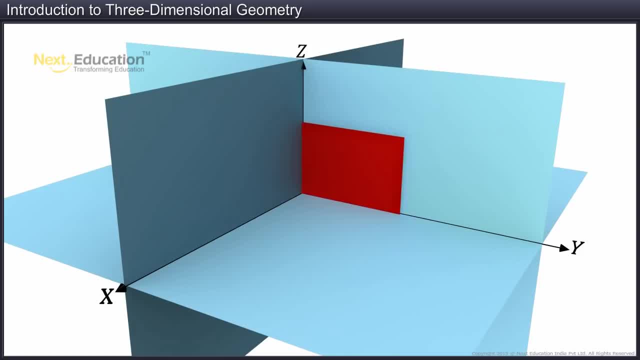 we will now locate a point using the intersection of planes. First, we will take a plane at a distance x and parallel to the yz-plane. Next, a plane parallel to the xz-plane and at a distance of y is taken. Finally, 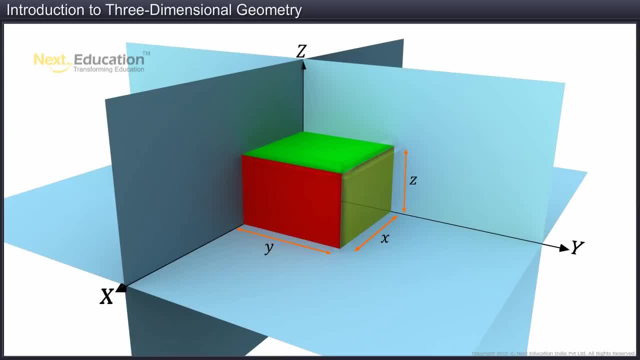 first, let's take two planes, one parallel to the yz-plane and the other parallel to the xz-plane. The intersection will be a line parallel to the z-axis. Likewise, the intersection of the other planes creates lines, as shown The concurrence of these lines. 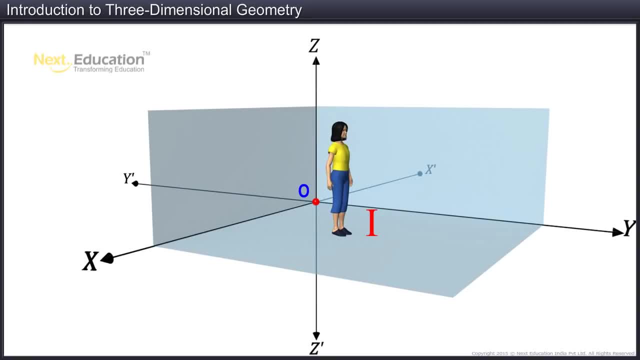 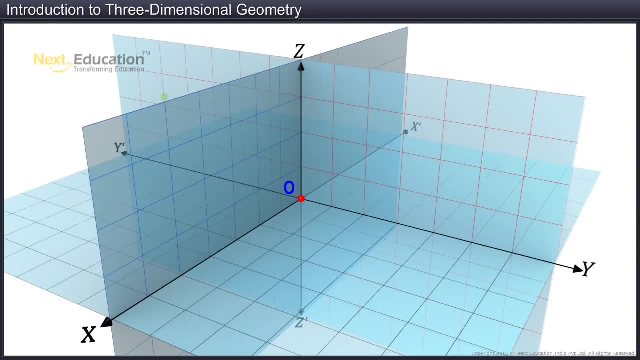 is point P. The coordinate axes divide the coordinate space into eight parts called octants. The sign of the coordinates determine the position of a point in a particular octant. For example, the point lies in the fourth octant, The x-coordinate. 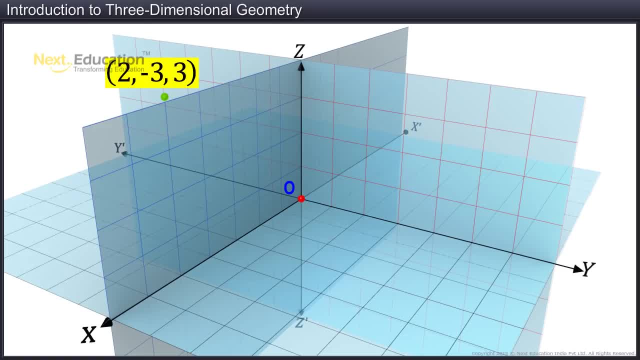 of the point is 2.. So we measure two units along the x-axis and mark a point. The y-coordinate is For this point. we measure three units on the xy-plane in the direction of OY' parallel to the y-axis. 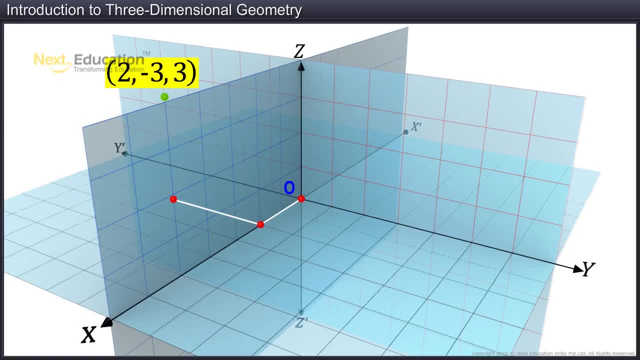 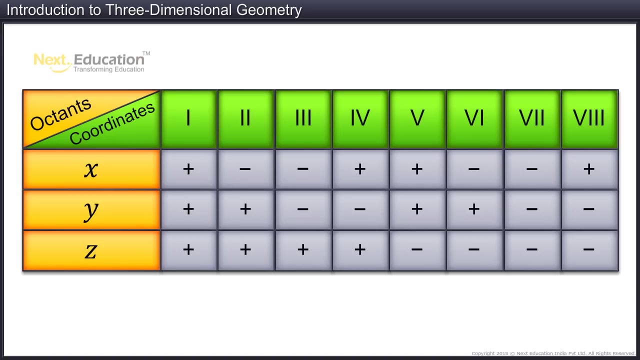 We mark a point there. For the z-coordinate, that is 3, we measure three units from the point perpendicular to the xy-plane. We can notice that the point lies in the fourth octant. The z-coordinate gives the details of the octant. 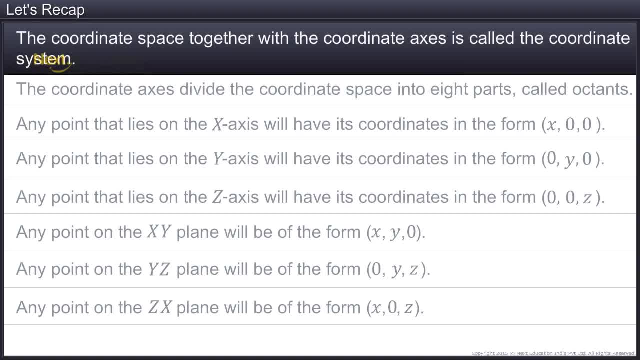 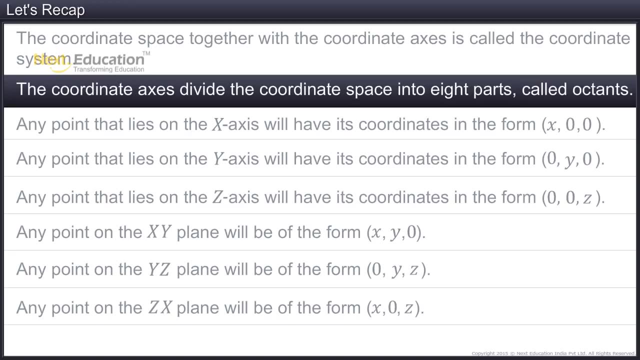 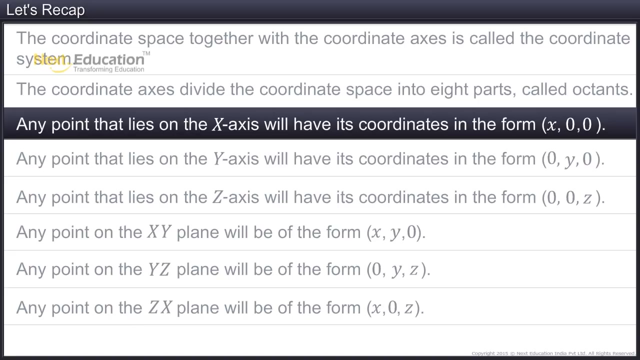 according to the signs of the coordinates of a given point. In this module you learned that the coordinate space, together with coordinate axes, is called the coordinate system. The coordinate axes divide the coordinate space into two parts: The point that lies on the x-axis. 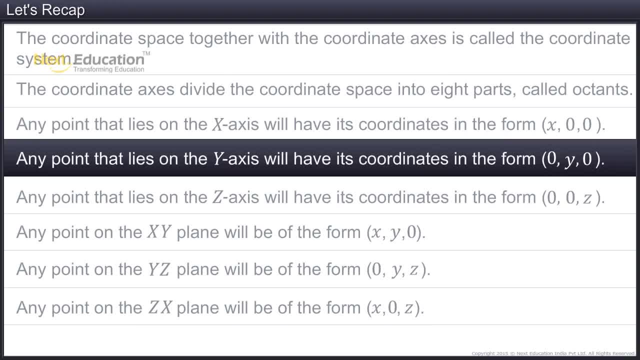 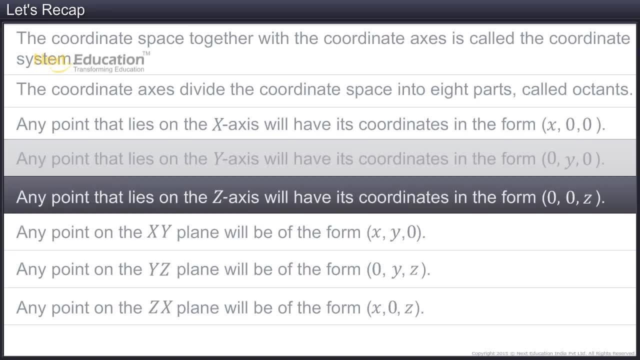 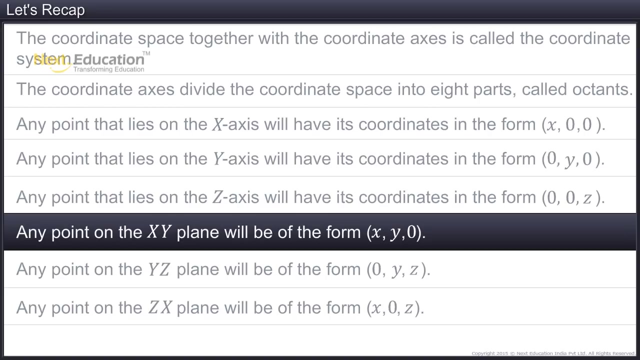 will have its coordinates in the form. Any point that lies on the y-axis will have its coordinates in the form. Any point that lies on the z-axis will have its coordinates in the form. Any point on the y-z-plane will be of the form: